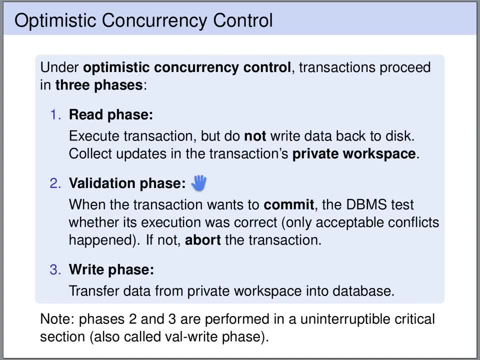 If not, the transaction will be committed. The transaction will be collected And if not, the transaction will be registered So we can run the transaction from here. The transaction will be collected, then this or another transaction will be aborted to resolve the conflict. 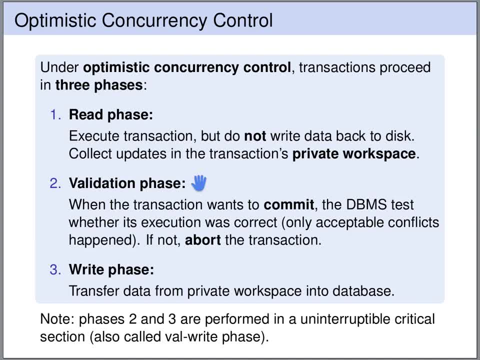 If the current transaction is not aborted, so the check succeeds. then we get to the write phase. then the updates of the transaction are written to the disk. They are made permanent in the database. The phases 2 and 3 are performed in an uninterruptible critical section. 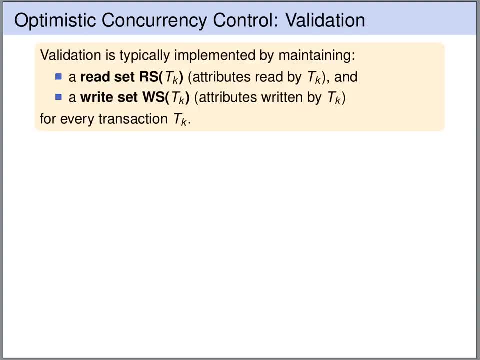 In optimistic concurrency control. the validation is typically implemented by maintaining a read set and a write set for each transaction. So the read set records what objects have been read by the transaction and the write set records what objects have been written by a transaction. 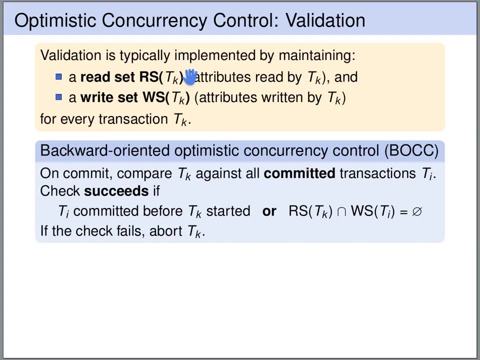 There's two flavors of optimistic concurrency control. There's a backwards-oriented optimistic concurrency control and there's a forward-oriented optimistic concurrency control. Let's start with the backward-oriented flavor In the backward-oriented, optimistic concurrency control. when a transaction, TK tries to commit. 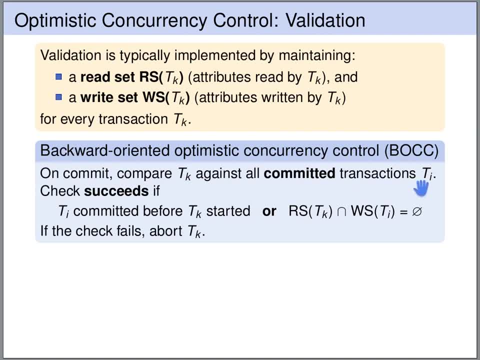 then we compare this transaction, TK, against all committed transactions, TI, And we check the following: We check whether TI has committed before TK has started. That's fine. So we go to the read set. We ignore all the transactions that have committed before TK has started. 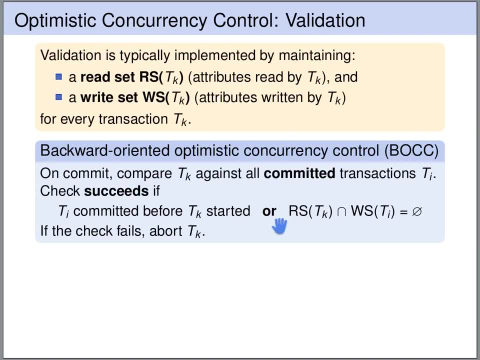 If TI has committed after TK has started, then we check the following: We check whether the read set of the current transaction has no overlap with the write set of the transaction TI. So what is the problem if there's an overlap? The problem if there's an overlap is TI has committed after TK has started. 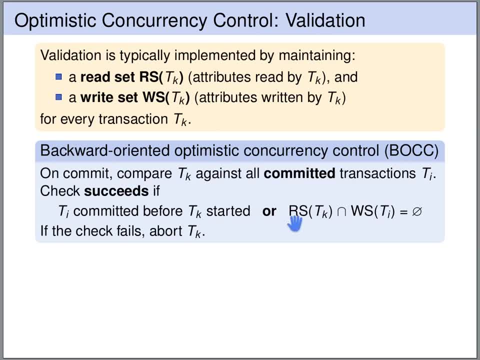 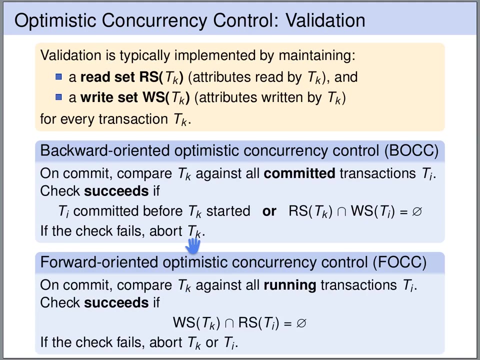 So that means that TK may have read an old value that has in meanwhile been overwritten by TI. So that's what we don't want. So if TK has possibly read an old value, then we have to abort TK In the forward-oriented, optimistic concurrency control. the check proceeds as follows: